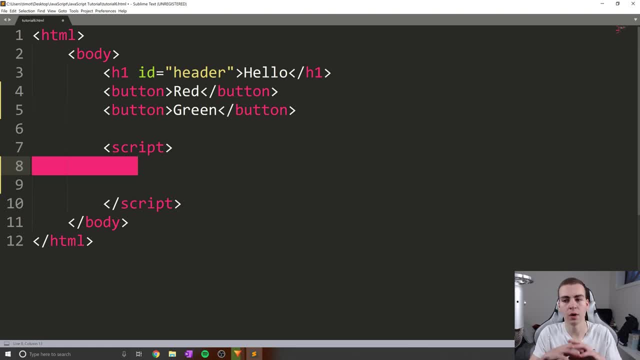 I say one thing. I don't really mean, you know, one line of code. I mean one overall operation. one overall function of your code is what it's performing. it's not, you know, messing around and doing 100 different things inside of it. Okay, so how do we? 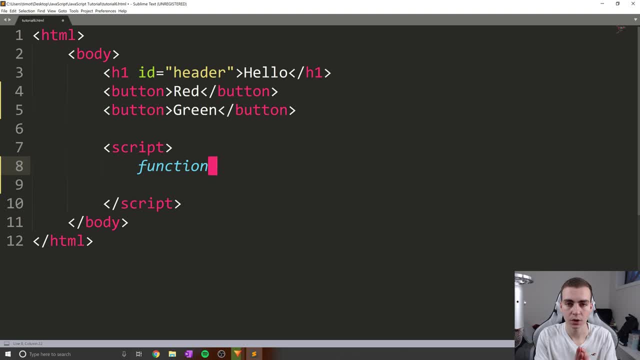 create a function. Well, to do it is actually pretty straightforward. we're going to type the word function, we're going to type a name- in this case I'm actually going to do a basic example before we get into the other one called add- and then we're going to put curly braces to denote. 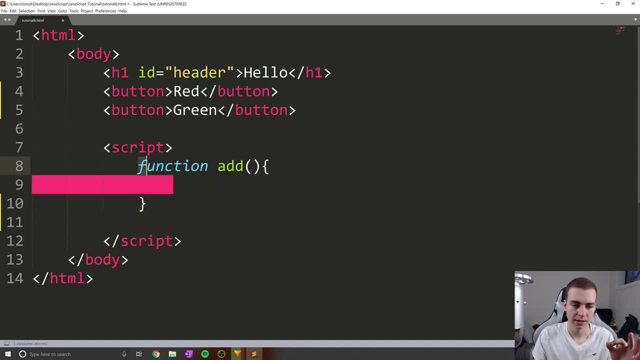 where our function actually is. So what I've done here is said: we're going to define a function called add, and anything that goes inside of these curly braces is what's going to be inside of our function. Now, to give you a really basic example, what I'm going to do is just console dot log. 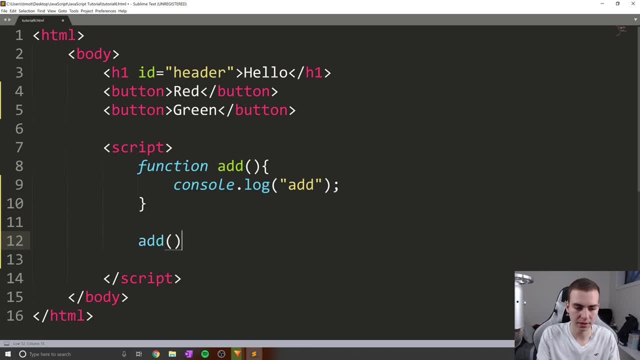 add like this, And I'm going to call my function by doing this: Now, I know you guys have no idea what's going on right now if you've never seen functions before, but let me break it down for exactly what's happening here. This is our function block, right? So this is the name of 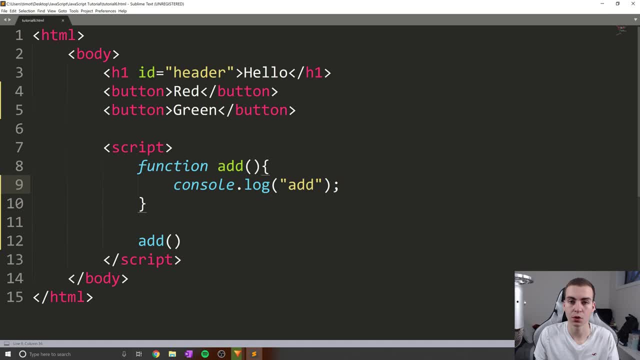 our function at this block of code- or any blocks of code for that matter- that goes inside of these curly braces will only happen when the function is run. So the function has to be run, we have to call the function and then whatever's inside of it will happen. So here, 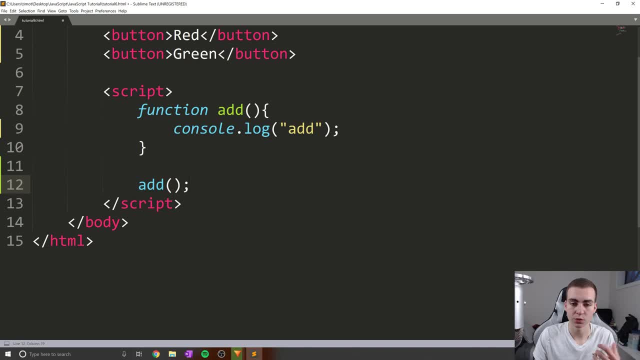 this is what we call our function call, And to call a function is really easy. all you do is type the name of it and then put two brackets at the end to say that you're calling it. So this is our function call, And essentially what's going to happen is when we're reading through our code. 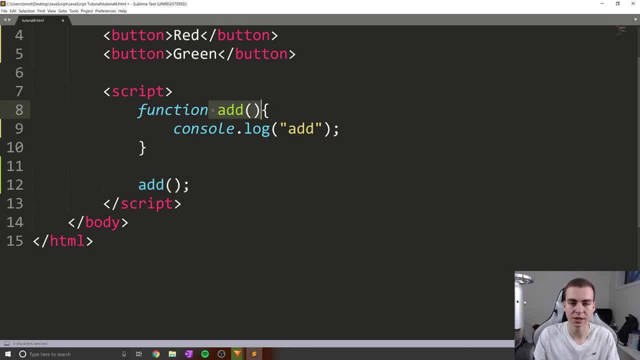 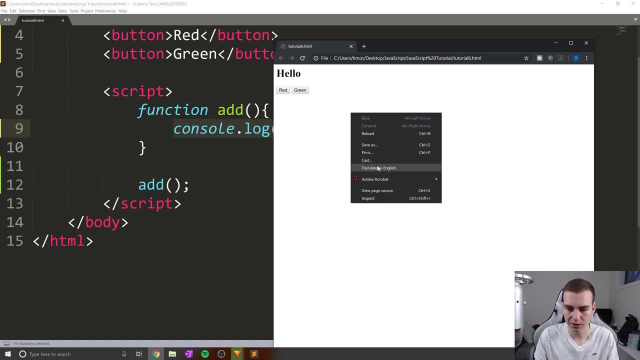 as soon as we hit this block, we're going to actually call this add function, which means it's going to run. So let me illustrate that to you by just simply running and refreshing this page. let me go to actually inspect element here And you can see if we go to. I got to find where. 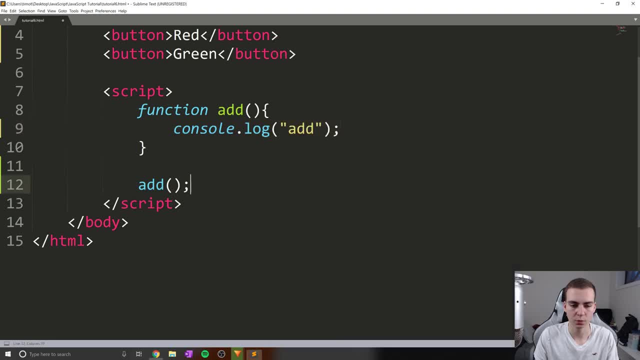 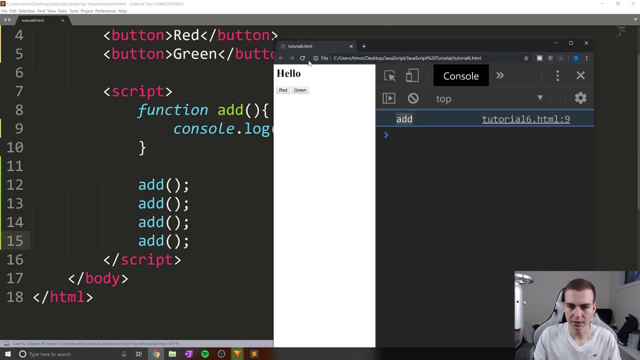 is this here console, we get add printed out to the screen. when I called add- And the great thing about functions that we can call them a bunch of times- So let's do this And you can see that now we have four ads popping up on the screen. So hopefully this is giving you an idea of why we 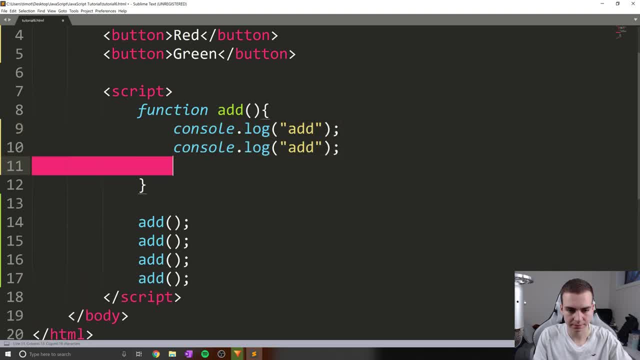 might use them Because, say, I wanted to print a sequence of I don't know, add 123 like that. well, rather than, you know, having to do this, I want to do this exact sequence of ads 100 times, rather than having to. 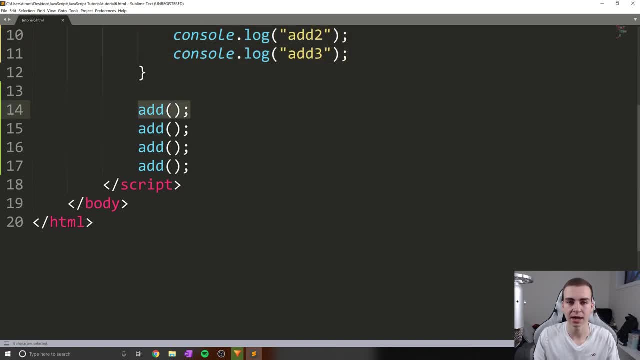 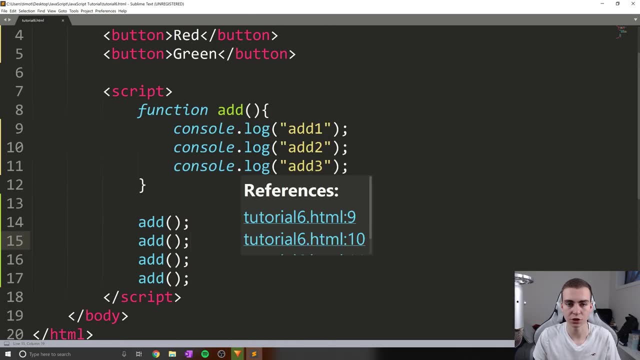 write 300 lines of code. what I would do is simply call add as many times as I want that to happen, right? So if I refresh this now, you can see we're getting all these popping up And that is. you know the basics of functions and why we use them so that we can reuse our code. So if you ever 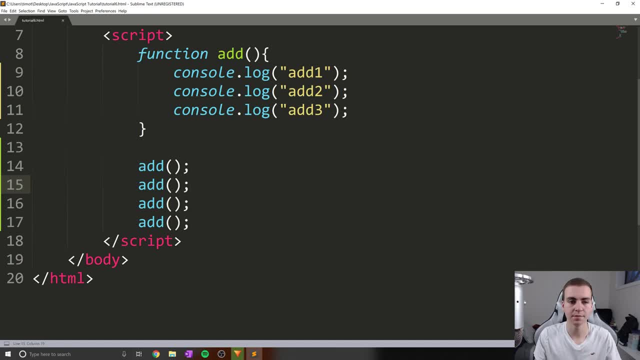 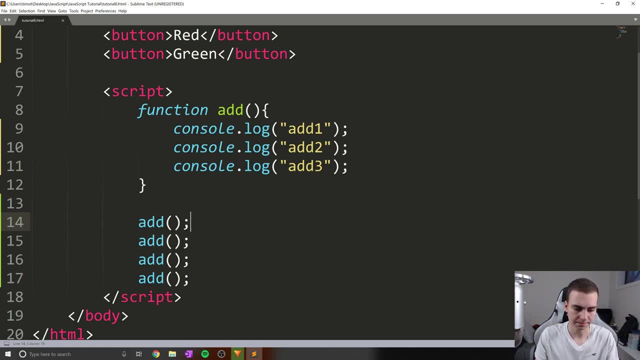 realize that you're writing very similar lines of code multiple times. maybe you just want to add them into a function And then you can just call that line of code once with one statement, rather than writing it a bunch of times. Okay, so let's go into a little bit more of a more advanced example here with add, And I'm going to 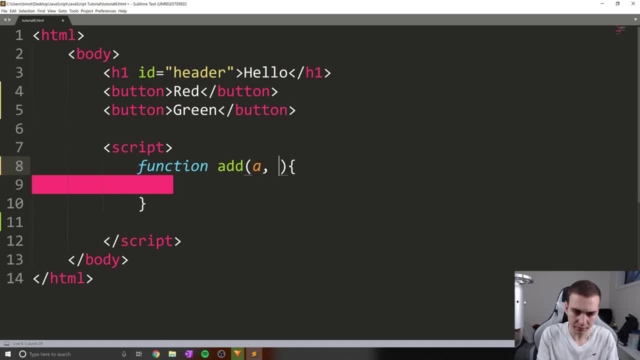 show you something called parameters and something called return statements. So what I'm going to do is I'm going to put two parameters in here. I'm going to call them A and B, And these are called parameters. Now, what these kind of stand for is the information that I need to pass to my function. 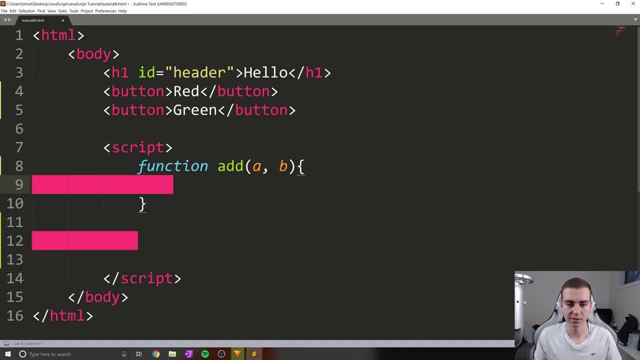 So this is the information that my function needs to be able to work, to be able to perform some computation. Now, in this instance, A and B are going to actually be two numbers that I'm going to add together, And what my function is going to do is take those two numbers, A and those number the. 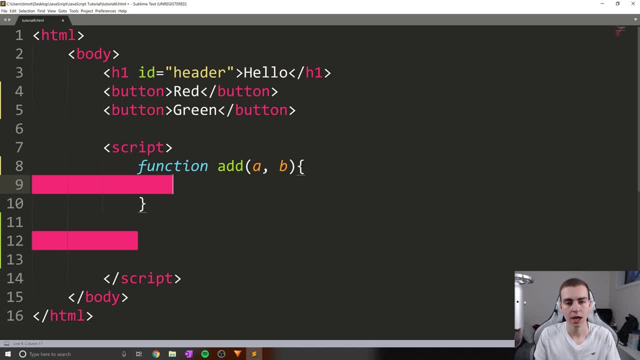 other number B, add them together and return the result to wherever my function was being called. Now, this might seem a bit confusing, but the examples are hopefully going to clear this up for you. So what I'm actually going to do in here is write a return statement. Now, a return statement. 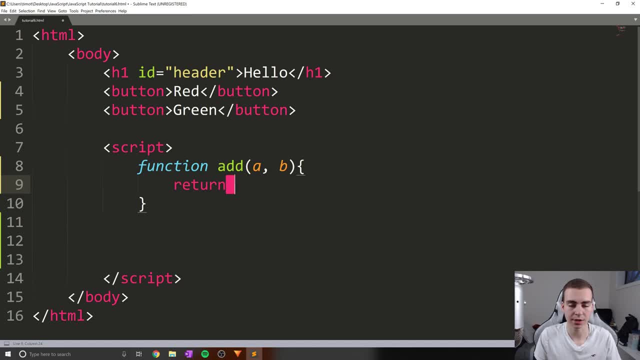 is different from logging something. I'm not printing something to the console. I'm returning a value, And the value I'm going to return is A plus B. Now I know everyone's confused. we'll get through this. what I'm going to do is create a variable here. I'm going to call it x. 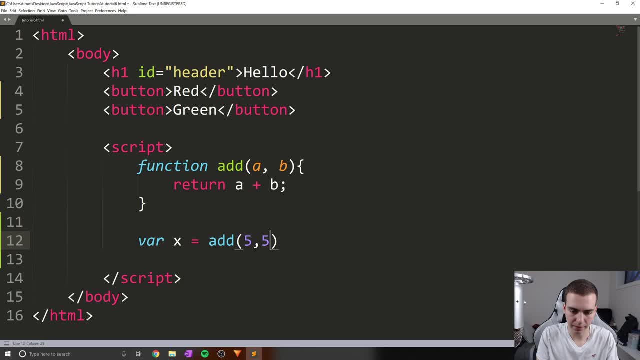 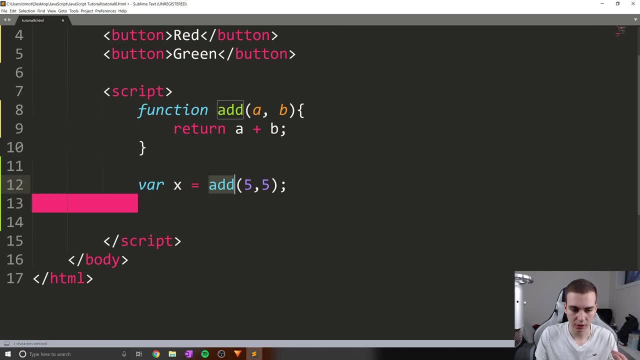 and I'm going to set it equal to add, And here I'm going to do five, five. Now we all know what five plus five is. we know that value is 10.. So what's actually happening here is, when I call add, I'm going to pass for the value a, the number five, I'm going to pass for. 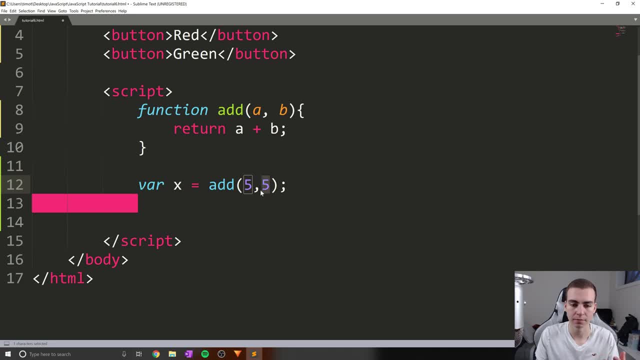 the number B or for the parameter B, the value five, Now what these are called our arguments. So these are parameters and these are arguments, And you can, obviously, you know I can- pass different arguments to them. I can say: var y equals five plus seven. right, I can do any numbers I want. 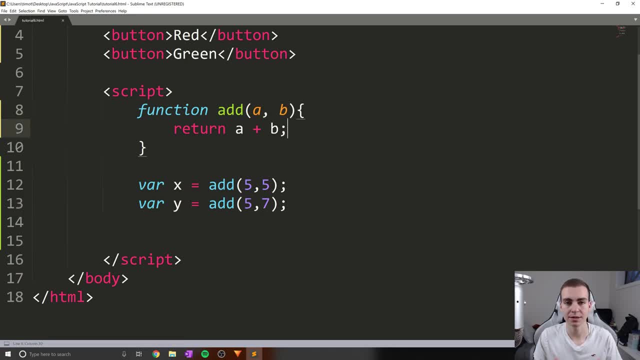 And this is the point of this- is that it can take any two numbers and return to me the addition of those numbers. So let's simply log out these values. I'm going to show you kind of how this works. So console dot log, we have x. 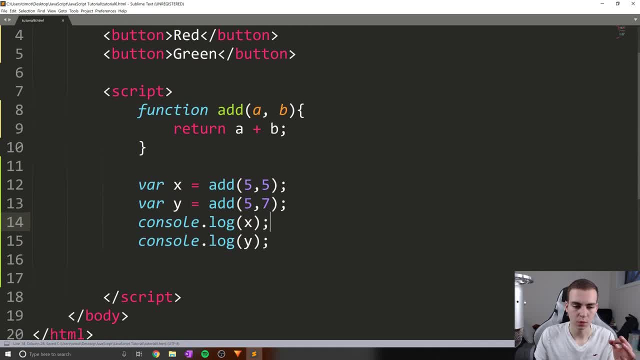 and we have y. So what's happening is, when we say var x equals, add five, five, what's going to happen is we're going to pass our values And then we're going to return the addition of those values. What this return is going to do is essentially say this line here that we've said: 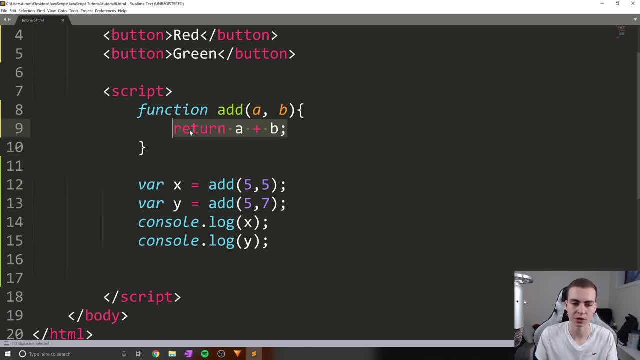 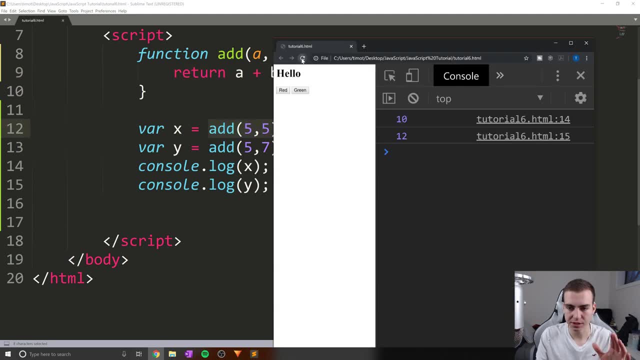 add five, five is going to be equal to whatever this return statement returns, which in this instance is 10,, which means that x should be equal to the value 10.. I know this might be confusing, but let's run this and see what we get. we get 10, and we get 12.. 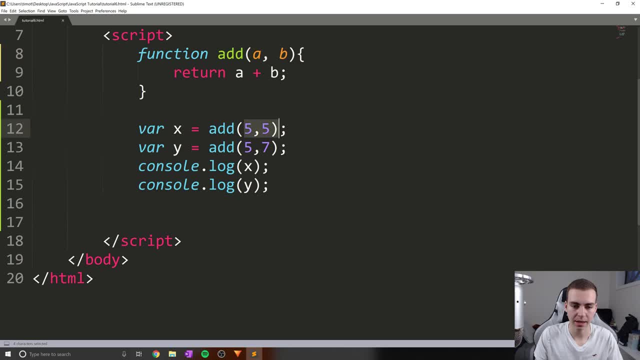 So what happened was we pass our values. you know, something happened. this gets replaced with whatever was returned from that function. So which is 10,, this one is getting replaced with 12.. And then we can print those two values out and say: you know, this is 10,, this is 12.. Those are answers. 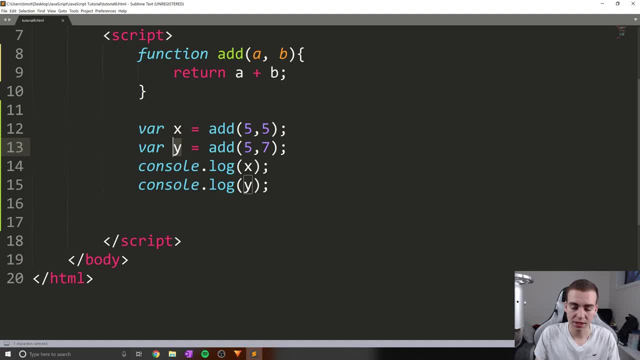 and we're storing them in variable x and variable y. That being said, though, I don't need to store them in a variable, And sometimes I don't want to store the value. I just want to, you know, use the value. So what I can do is actually do something, like you know, 234, and like negative. 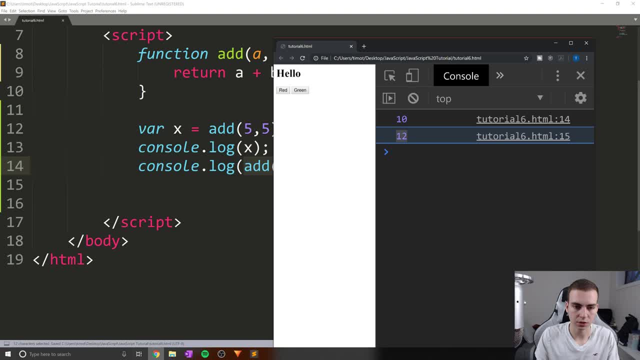 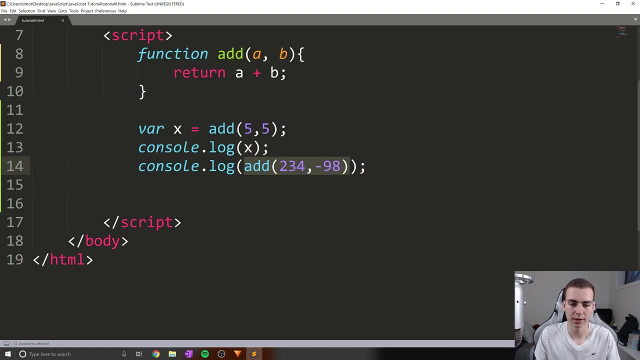 90, eight. maybe let's pass that in here And I can log the result of that addition. So here you know, we get our value 136,. I'm not storing it in any value, but I can still show it, because what happens? 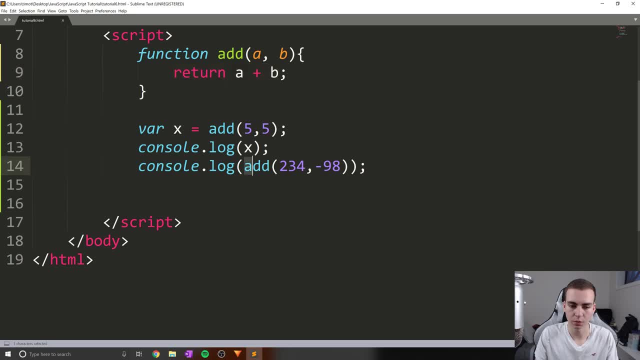 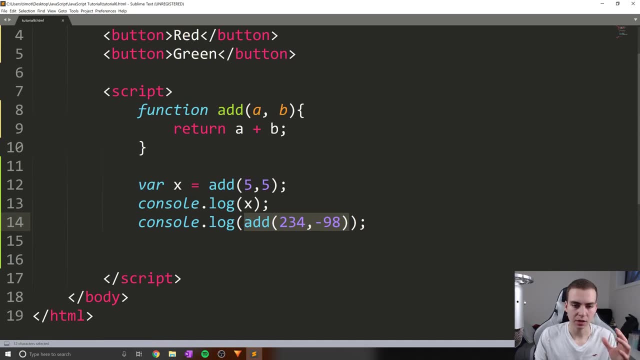 is when I call this, the return statement is going to whatever returns will replace this line, And then you know we can demonstrate that and show that on the screen. Okay, so I think that is the basics. I've shown so far, that you know we can have a function that has parameters, we can have a 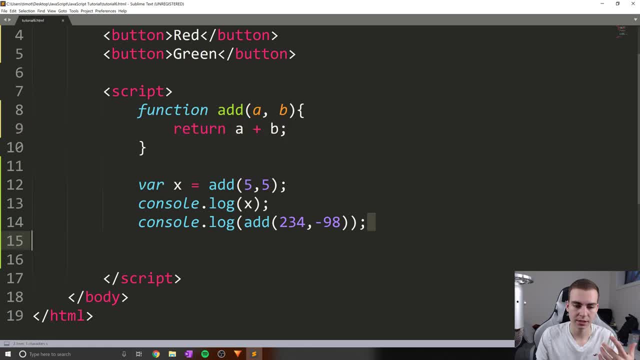 function that doesn't have parameters. we can have one that has returned, and we can have one that doesn't have a return. What about a function that has parameters but doesn't have a return statement? Well, that's more than fine. I could do something like console dot log a plus B. And then if now, if I call my add. 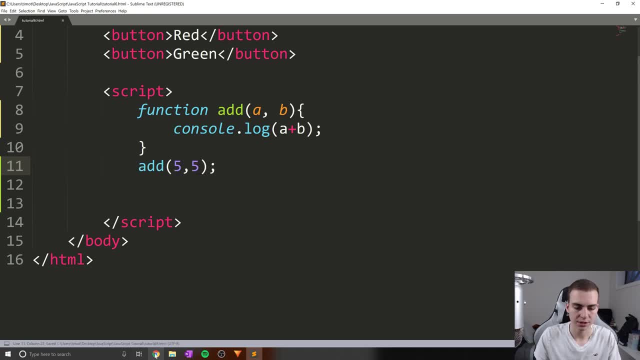 function, and I do five, five, watch what's going to happen. So we're going to print the value 10.. Why does this work? Well, same thing as before. we have our parameters a and B. what we've done is: 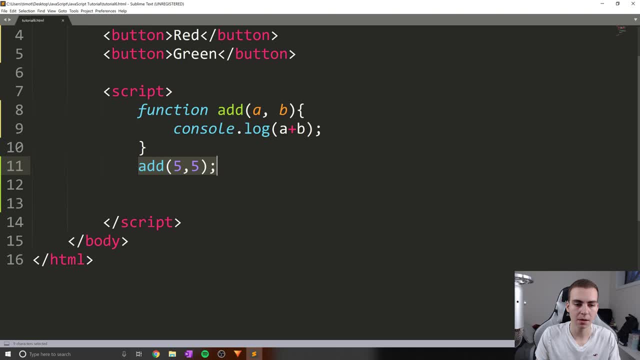 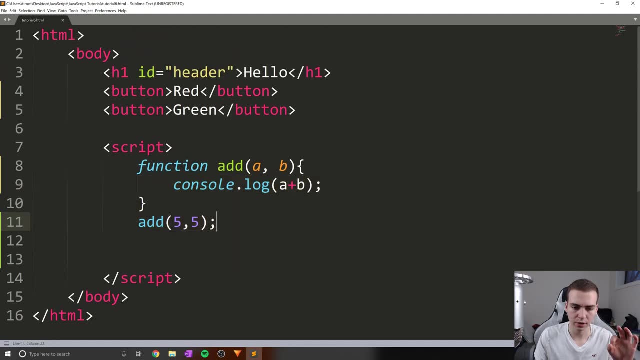 we've called add notice. we're not printing anything down here, But what happens is inside of the function we print the addition. So obviously that's going to work fine, And you know that is how this works. Okay, but now how about some of the more cooler parts of functions that I want to get? 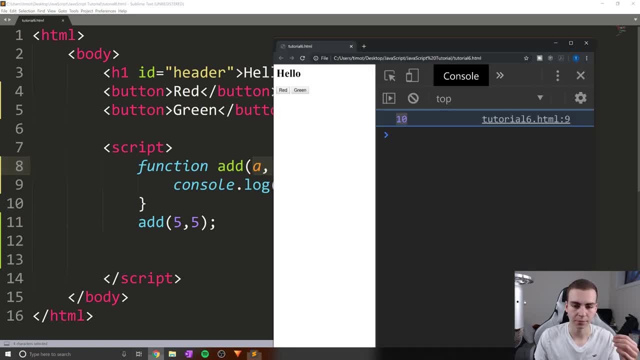 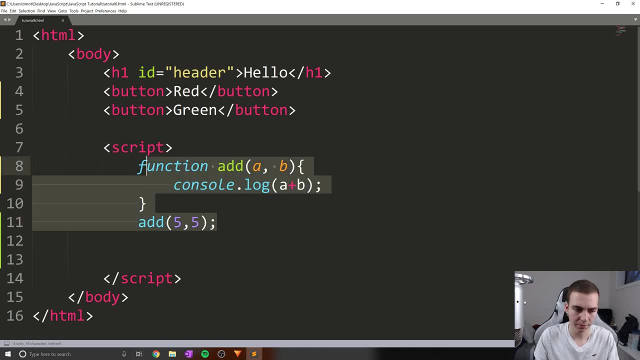 into and then finish in the rest of the video. How do we call a function from our HTML? like I want to press this button and I want to call a function, How do I do that? Well, let me show you So what. 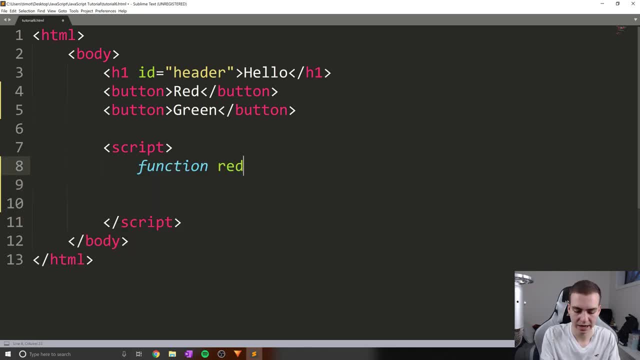 I'm going to do is actually create a new function And I'm going to call this function red, And all I'm going to do right now is simply say console dot, log- red. Now, inside of my button tag, what I can actually do is set the function that I want to trigger when 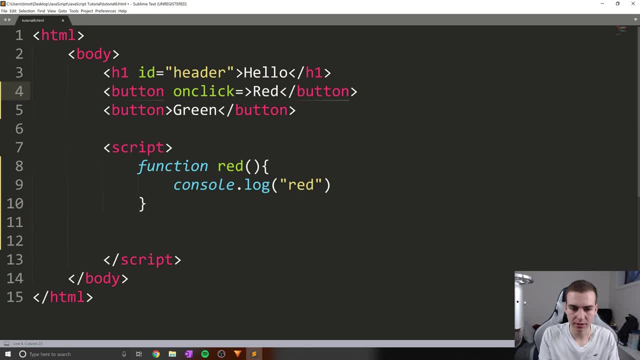 this button is pressed And to do that, I simply say on, click equals and in this case, red. Now, what this is defining is essentially, when I click the button, I want to call the function, which is called red, which obviously is right here. So let's see this and see if this works. Give this a. 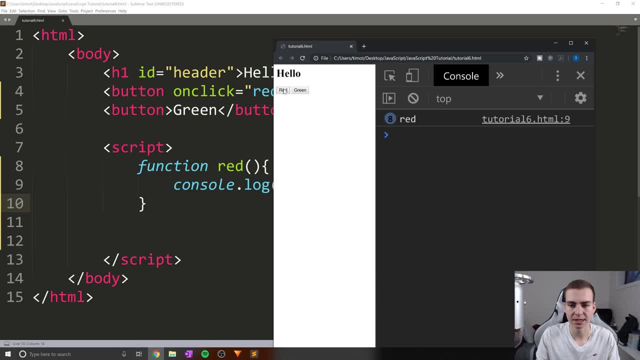 refresh. When I click red, you can see that red is printing out to the screen. And notice, you know. obviously it's keeping track of how this function works. So let's see if this works. And now let's give it a try. If I click red, it's going to fill up as if this was this nextще function. 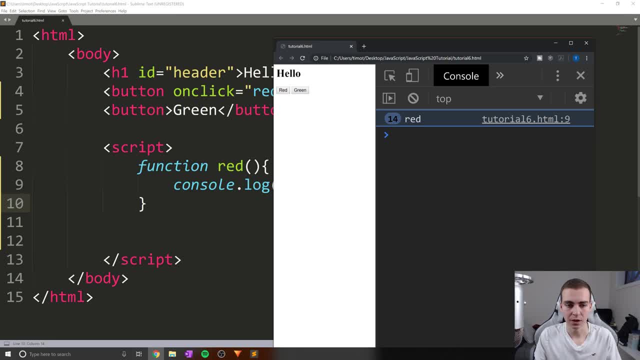 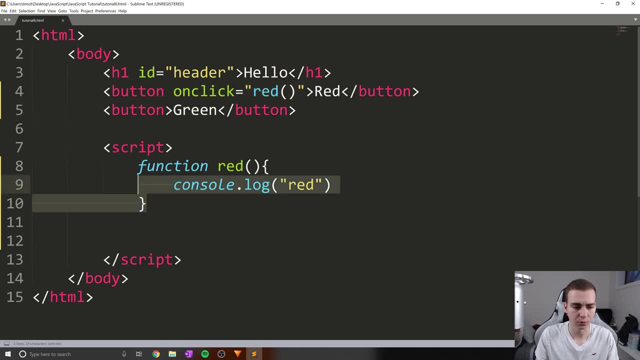 however many times I pressed it, just to tell you that same output showing up. And that is as easy as that is to do. If you want to call function from your JavaScript, you literally just put in quotation marks- whatever the name is inside of HTML, sorry, and we'll call that function Now. 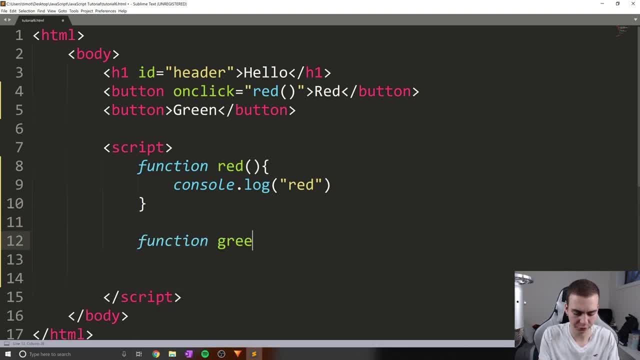 let's do the same thing for blue or green or whatever I have. Okay, so it's called this green, And let's do console dot log Green. and I keep forgetting my semicolons, but I guess I don't even need. 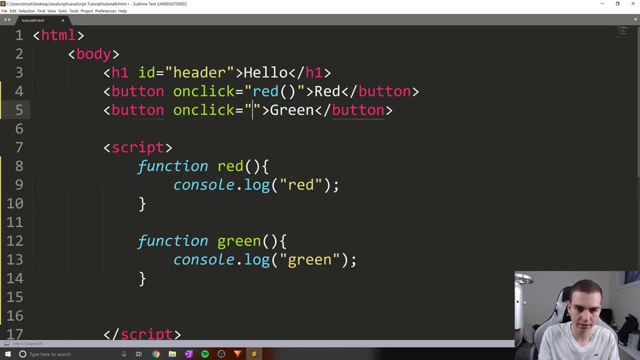 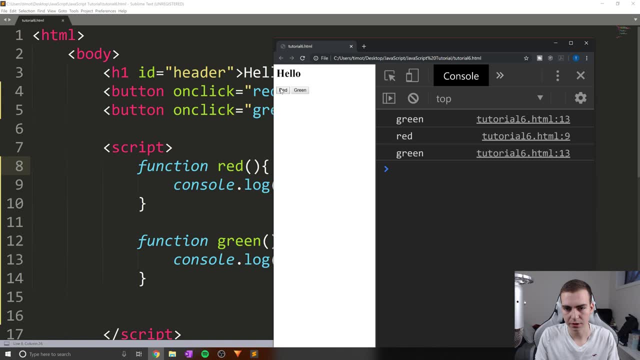 even need them anyways, but I just like to add them, So let's do on: click equals green. Okay, So let's run this now: Refresh: green, red, green, red, green, green, green, green, green, red, red, red. 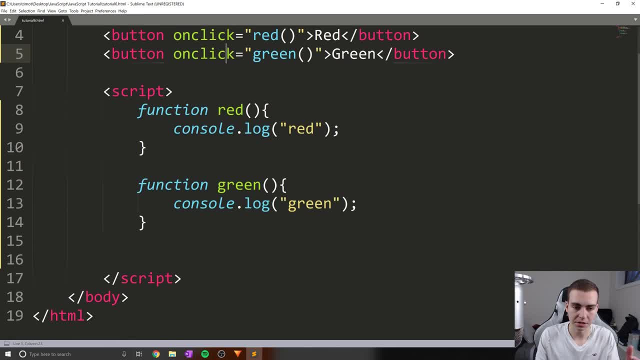 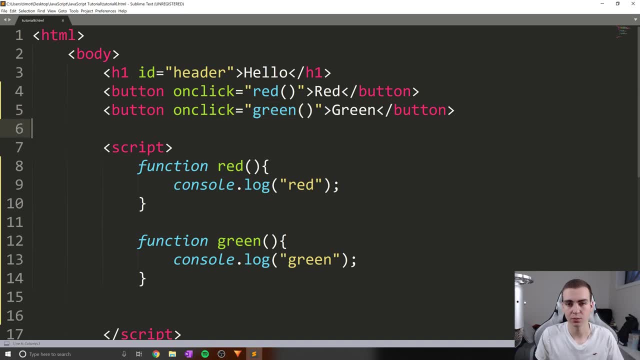 See, and that is exactly how this works, And that is, I mean, pretty cool in my opinion. Now, what you guys can do is have buttons And when you press them, you can trigger some JavaScript, which is just the start of the. 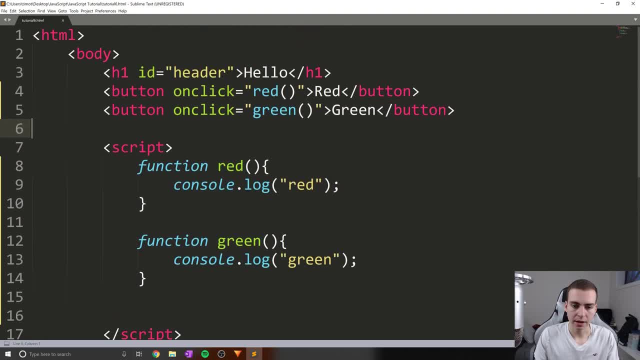 really cool things we're going to be able to do later in the series. Now, what I said, though, was: I don't want to just console that log. I actually want to change, you know, this element I want to change. Hello, Well, we. 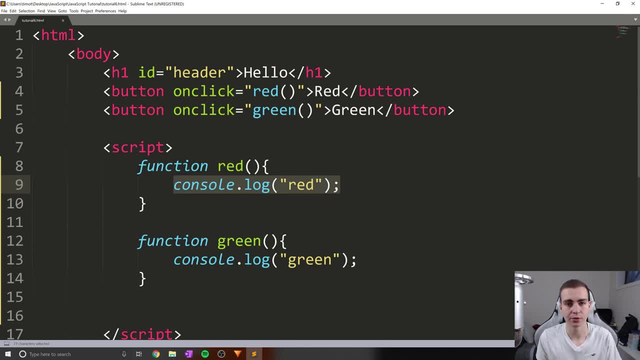 actually we know how to do that right. We know how to change- maybe not the color right now, if you haven't seen that command- but we know how to change the value of our H- one tap. So how do we do? 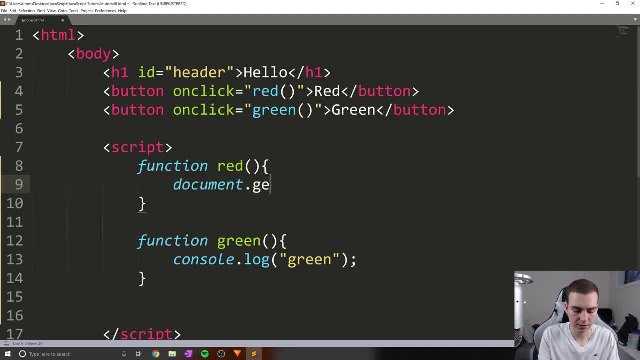 that. Well, let's do one in here: document dot, get elements. If I could type properly by ID- don't know what's going on with my keyboard here- Let's do header as our ID And then we're going to do. 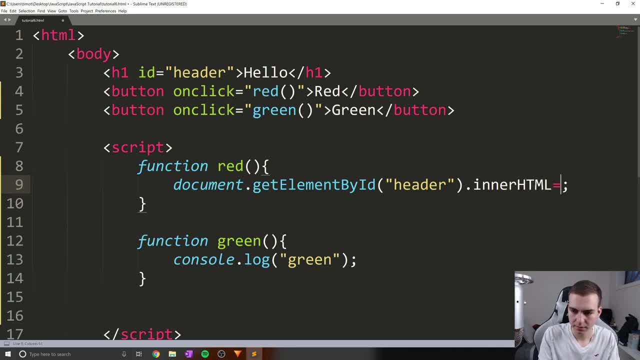 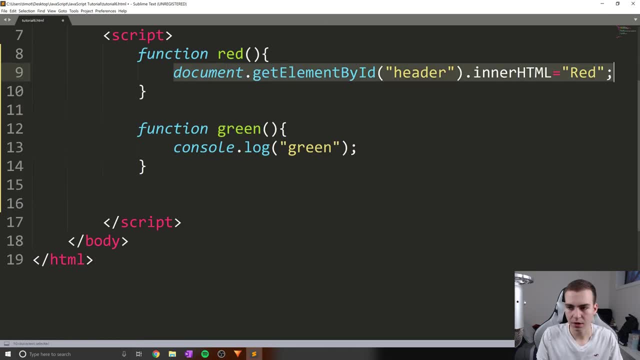 what is it? dot? inner HTML equals. What should we do? Let's actually just make this red for now. Great. Now let's do the same thing. I'm going to copy this to save us the pain of typing that again- and let's put in green So. 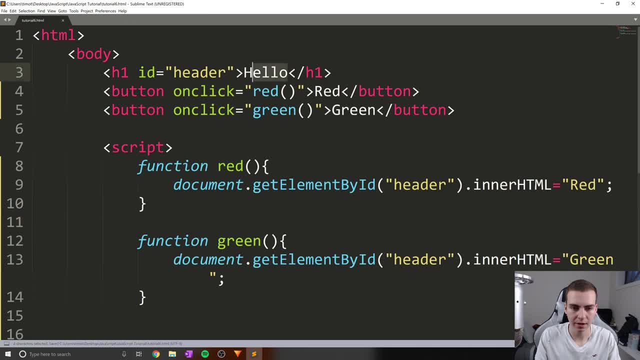 I haven't changed the color yet. What I'm actually going to be doing now is changing the value of this header tag to be either red or green when I press one of these buttons. So let's see if this works or if I mess something up. let's. 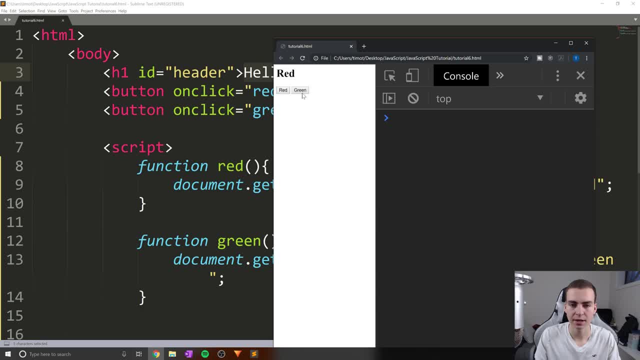 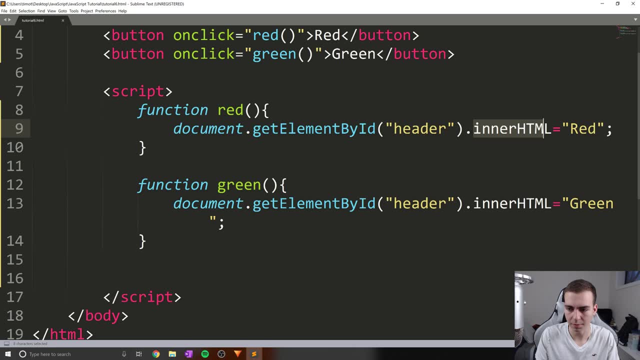 refresh. When I click red, you see it changes to red, And when I hit green, it changes to green, And that is, you know as easy as it is to do this. Now, what if we want to change the color? Well, I'm going. 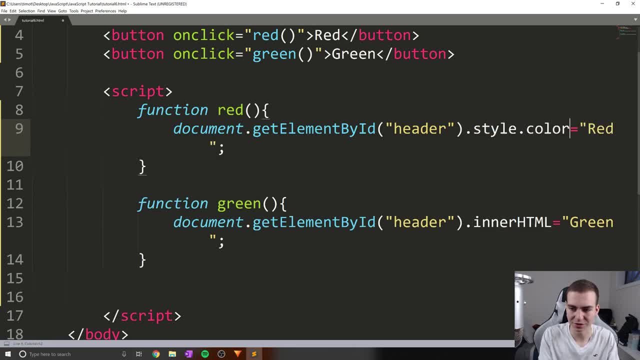 to give this a shot, because I always forget how to do this, but I think it's something like thought style dot color, And I'm pretty sure this will actually change our color to be either green or red, Although I don't really know, but we'll give it. 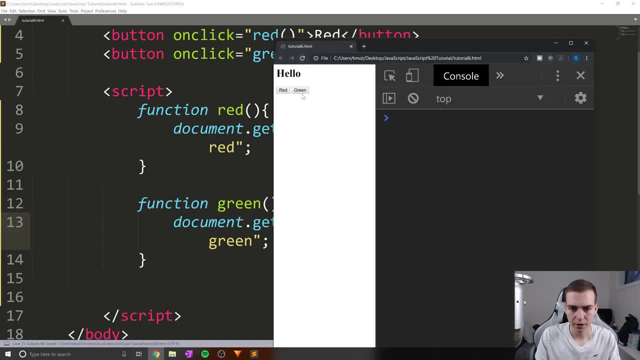 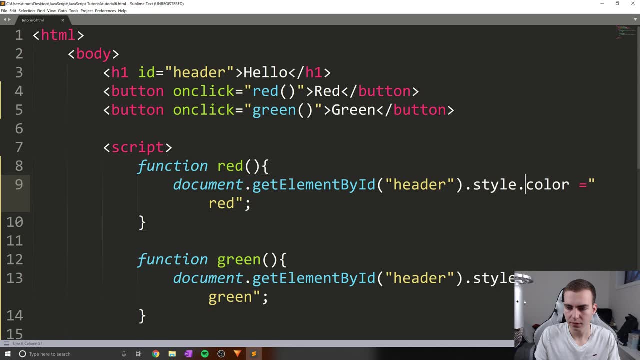 a shot, Okay, So let's run this fresh. when I press this, Oh, there we go: Our color is changing from red to green. So to do that, what I did was dot style, dot color and change that to lowercase red and